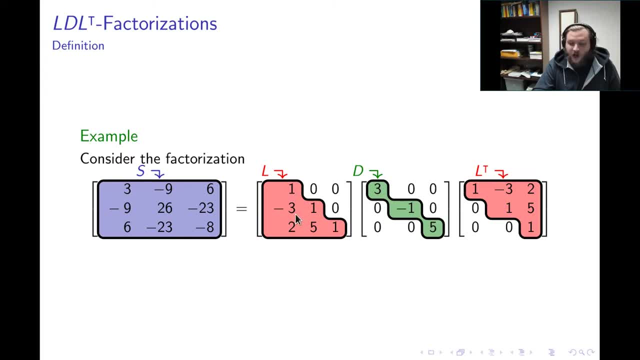 So, as we can see, L here is a lower unitriangular matrix. That means it's a lower triangular matrix with ones on the diagonal. D. here is a real diagonal matrix. so the only places where there aren't zeros in D are on. 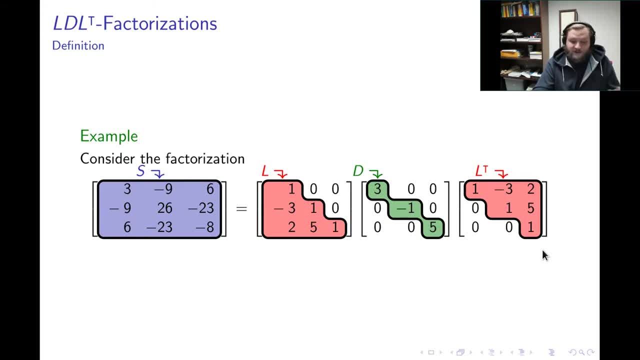 the diagonal And then L transpose, of course, is the transpose of L, And one of the things that we want to do here is we want to make sure that we have a real symmetric matrix. So once we have this factorization, of course, that forces S here to be real symmetric, which 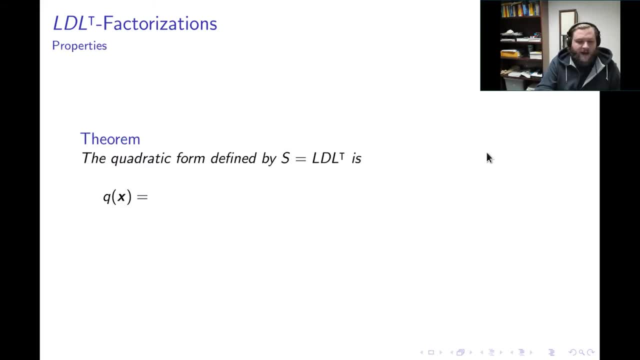 if we look at it, of course it is. Now, what's the point of studying L, D, L transpose? Well, if S is real symmetric, that means it defines a quadratic form. The quadratic form is the inner product of the input vector X, with L times, D, times L. 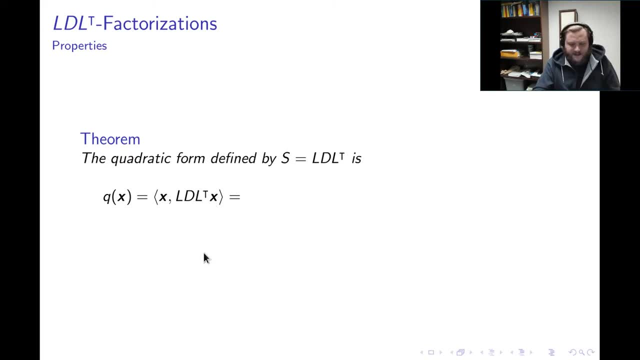 transpose times X, And we've seen things that look like this before. When I look at this, I kind of see an unbalanced matrix. I see an unbalanced inner product, So I like to move the L to the other side using the adjoint property of inner products. 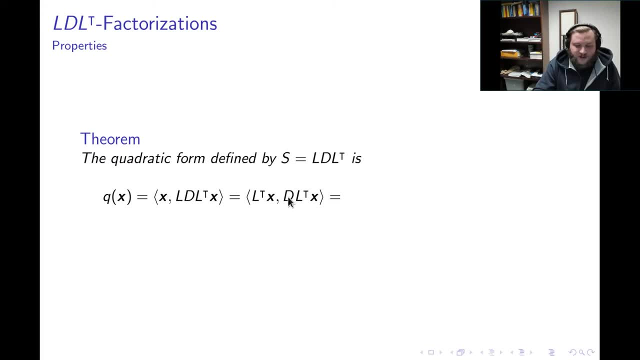 And that gives me L transpose X inner product with D times L transpose X. So now I can change variables much like we did when we completed the square using the spectral theorem, except this is a totally different factorization. This is now if I set Y equal to L transpose X. I'm now looking at the inner product of. 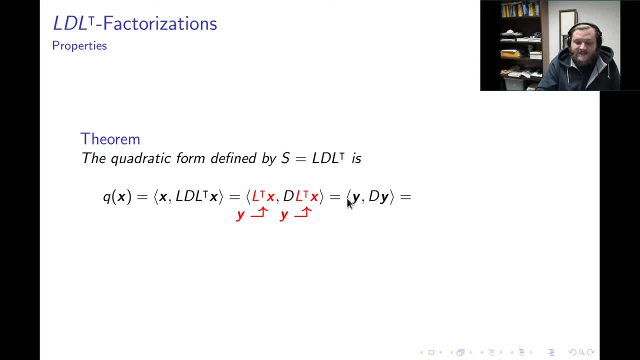 Y with D times Y, And the nice thing about this expression is that I can now write this as a linear combination of squares, where the coefficients are the diagonal entries of D and the squares are the coordinates of Y, which is L transpose times X. 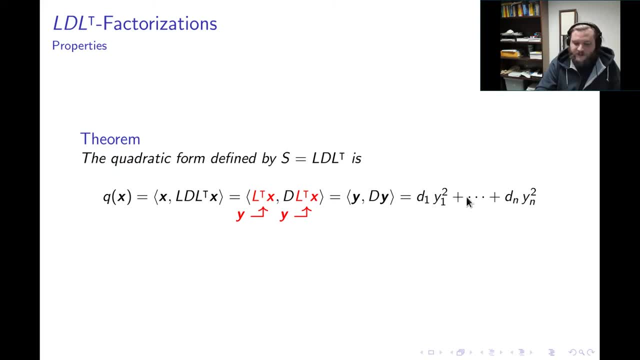 So this is D1 times Y1 squared, plus D2 times Y2 squared, plus Dn times Yn squared, where these Ds are coming from the diagonal of D And the Yn is coming from the diagonal of D And the Ys are the coordinates of L. transpose times X. 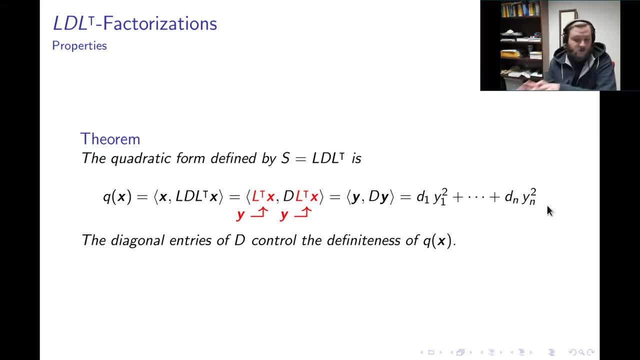 And so, of course, once we have this expression again- much like in completing the square, except this is now totally different- what we see is that it's the diagonal entries of D that control the definiteness of this quadratic form. So all we have to do is look at the signs of the diagonal entries of D and that automatically. 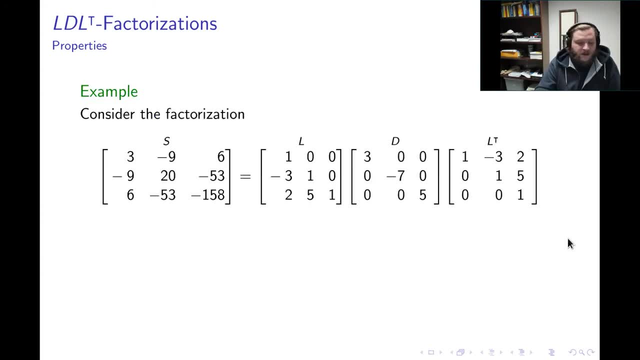 tells us what the definiteness of the quadratic form is. Let's look at an example Here. I have a real symmetric matrix S factored as L times D. If I look at the quadratic form defined by this real symmetric matrix S, I take advantage. 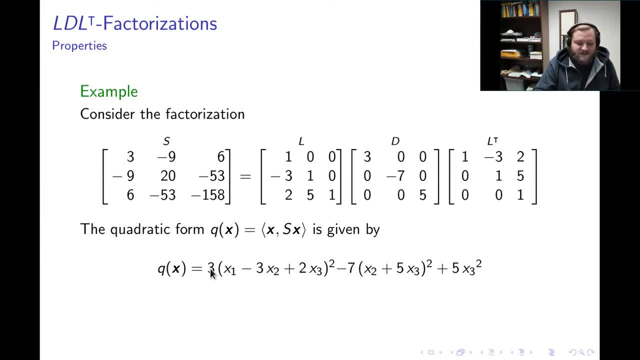 of the calculation we just did and realize that this is D1 times Y1 squared, plus D2 times Y2 squared, plus D3 times Y3 squared. What are those specific entries? Well, D1 here should be the first diagonal entry of D, which is 3.. 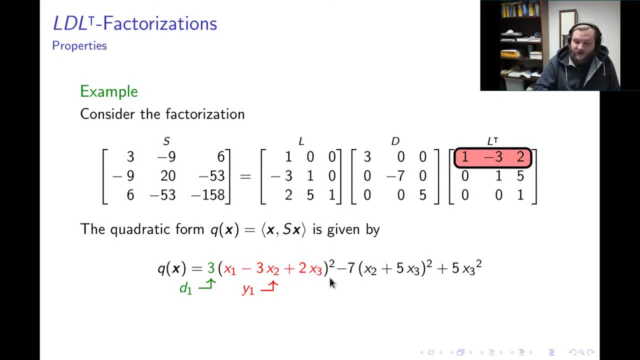 Y1 should be the first coordinate of L transpose. The first coordinate of L transpose times the input vector X. If I multiplied L transpose here by X1, X2, X3, the first coordinate would be 1 times X1 minus 3 times X2 plus 2 times X3.. 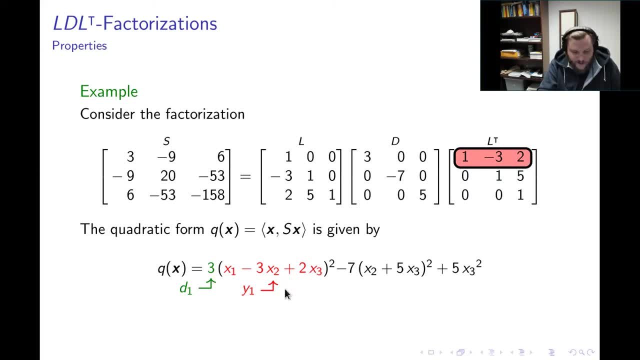 So that's my Y1 here. So my first term is 3 times Y1 squared. The next term should be D2, which is the second diagonal entry of D. that's negative 7, multiplied by Y2 squared, And Y2 squared or Y2 would be. let's see if I look at the second row of L transpose. 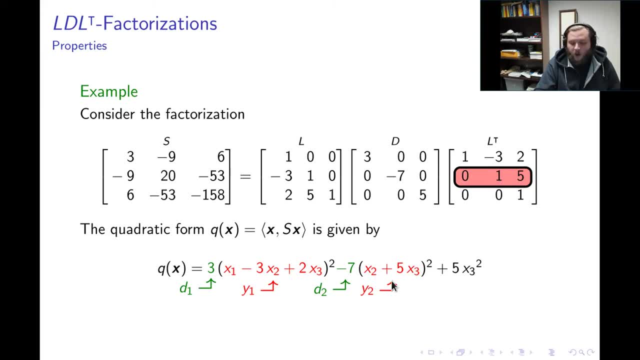 that should be X2 plus 5X3 quantity squared. now, The last term here should be the third diagonal entry of D, which is equal to 5, multiplied by Y3 squared. Well, what is Y3 squared or Y3 here, equal to. 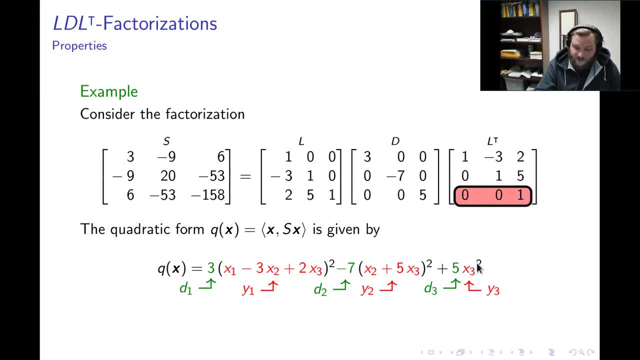 It should just be equal to X3.. So now I get X3 squared, So I have a nice way of presenting this. So I have a nice way of presenting this quadratic form as a linear combination of squares, And what I see in my coefficients is a mixture of positive and negative numbers. 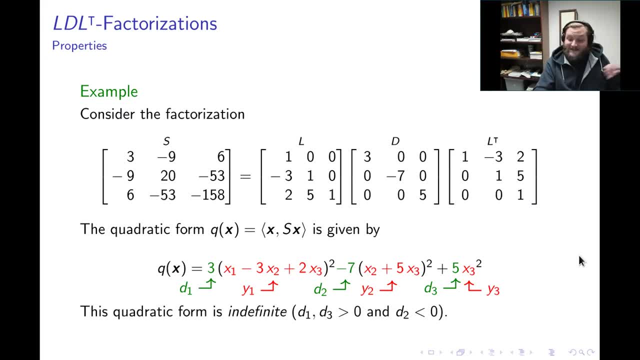 So that tells me that the definiteness of this quadratic form is indefinite. Two of the diagonal entries of D, D1 and D3, are positive, that's 3 and 5. And the middle one, D2, is negative. 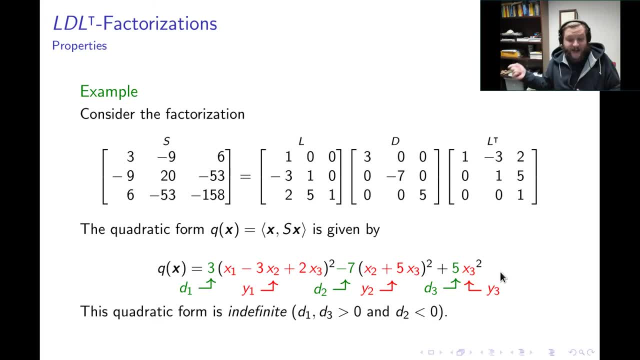 So sometimes this quadratic form is positive, sometimes it's negative, which means this is an indefinite quadratic form. So if I have L times D times L, transpose, I can quickly infer the definiteness by looking at the diagonal entries of D, And the reason that I can do this is because I have this.